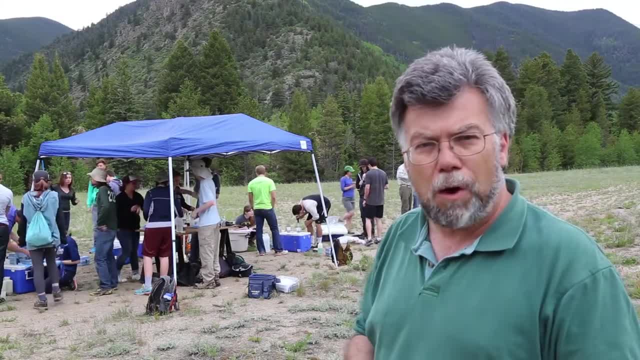 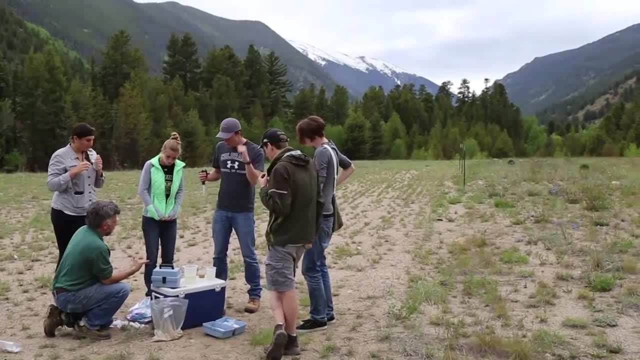 have to do some chemistry, They have to be able to measure them. They've got some metals in the water, So they'll take these samples back and tomorrow in the lab we'll run something called ICP which will give us copper, zinc, lead, those. 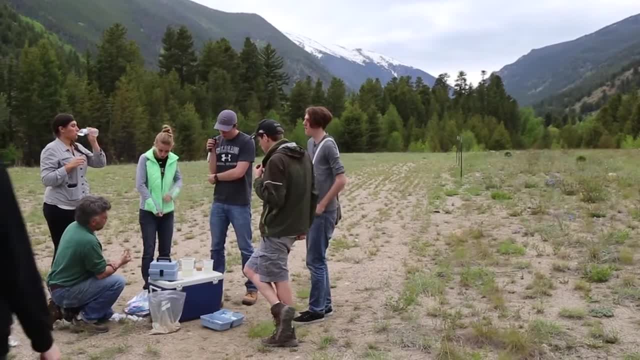 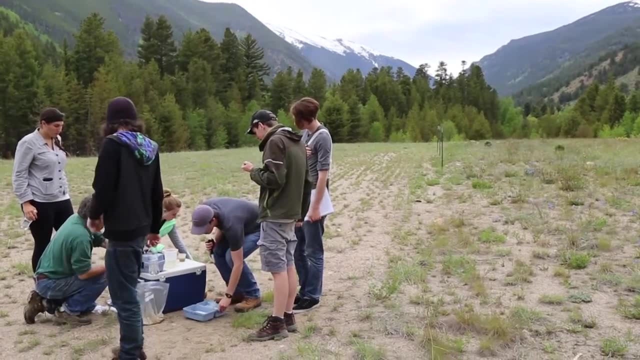 sorts of things. They also need to know things like the pH and the conductivity of the water. So they've got some field kits set up and they have some other experiments that they can measure, do measurements in the lab or in the field here as well. So they're pretty. 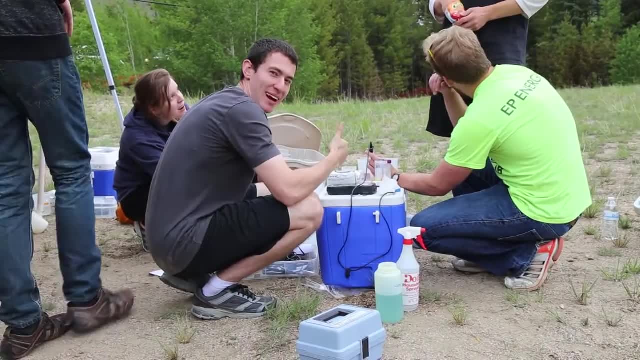 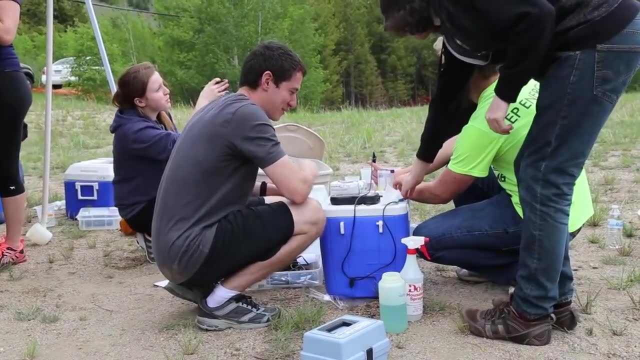 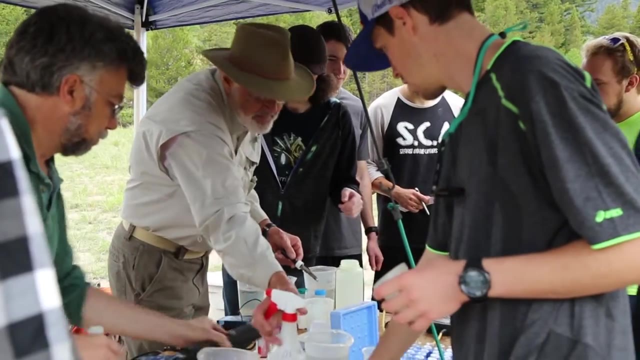 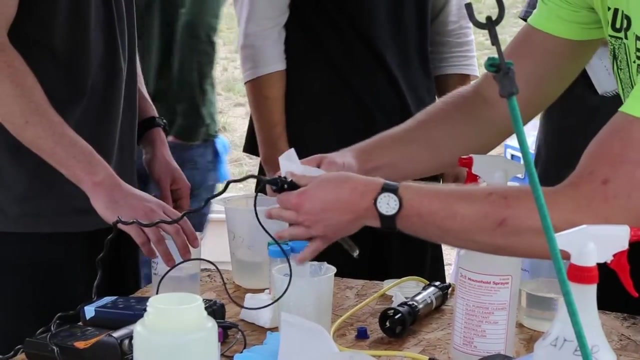 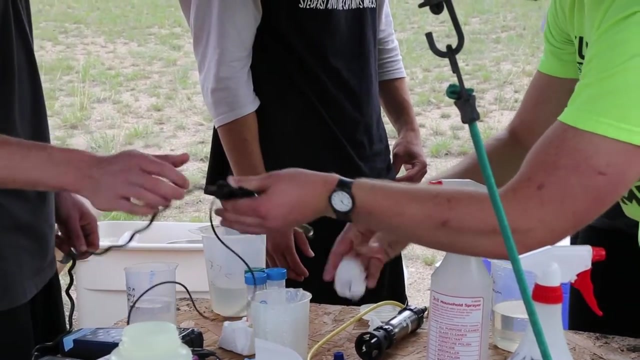 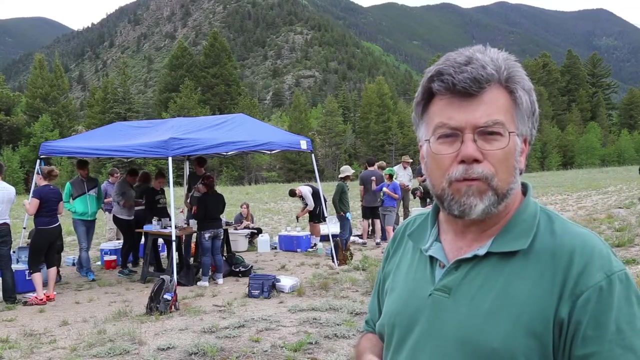 busy and we've got four or five different objectives and each class or each group has a slightly different objective In the spirit of a field session. I don't know how many of these guys are going to wind up going for environmentally oriented water. 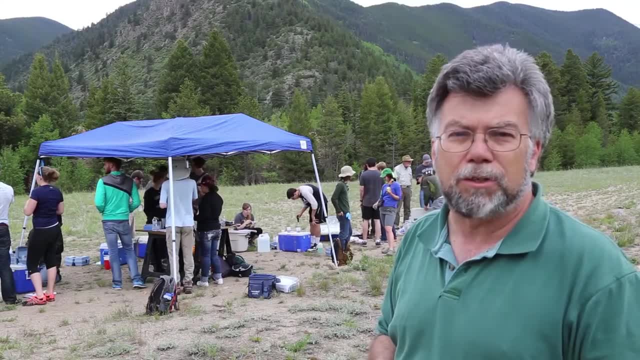 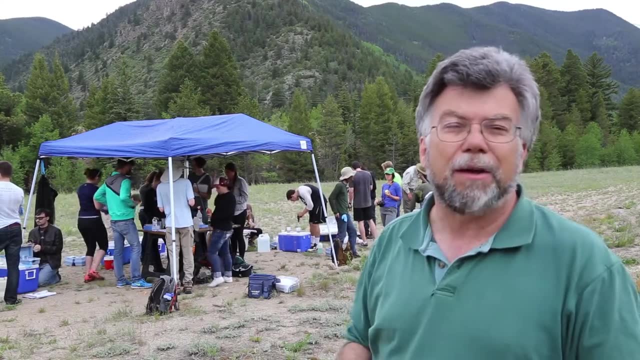 They're going to get jobs, but certainly this is the kind of stuff they might encounter once they're done with classes- is if they want to go into environmental consulting or some other areas. Having these field skills, knowing how to do some of the very simple. 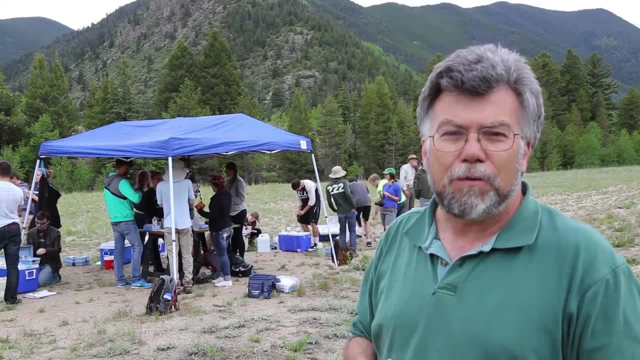 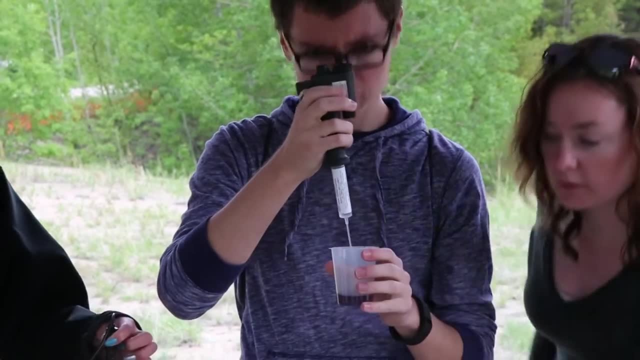 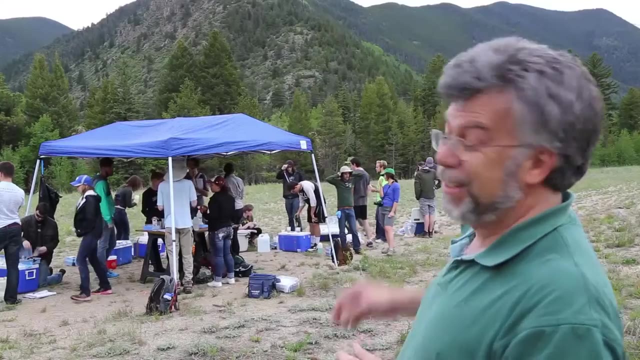 things that really become fairly difficult in the field. you know, just filtering a sample, just measuring a good pH of the sample- all that's a little bit harder in the field, And so it's good to have this experience. As you can see, it's a water-based system. 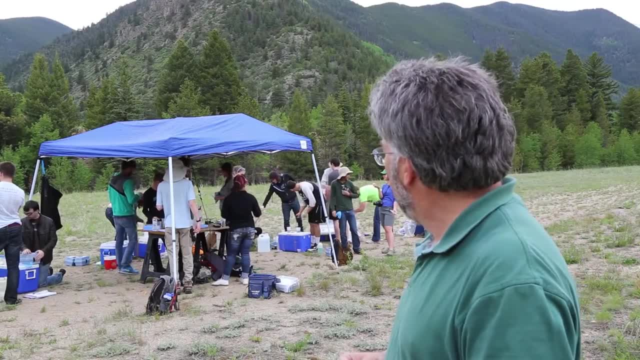 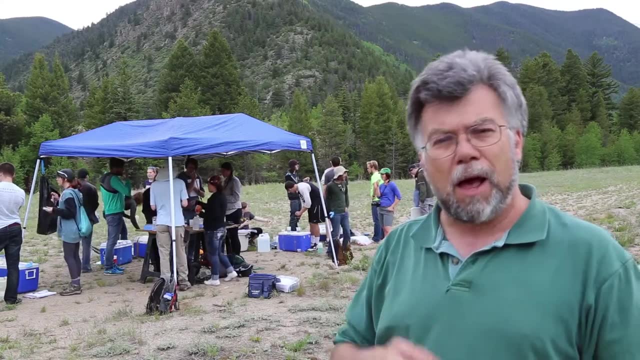 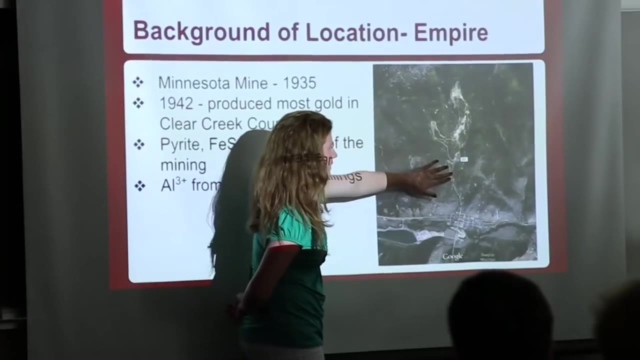 It's controlled. chaos, is what I like to think, And so again, we do this type of practical work out here, but again, we try to tie it back to the basic chemistry that they did in the lab. Now, what happens tomorrow is we're going to have a bunch of data to look at. We're 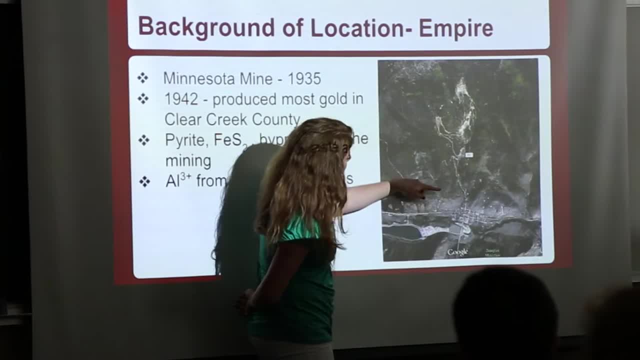 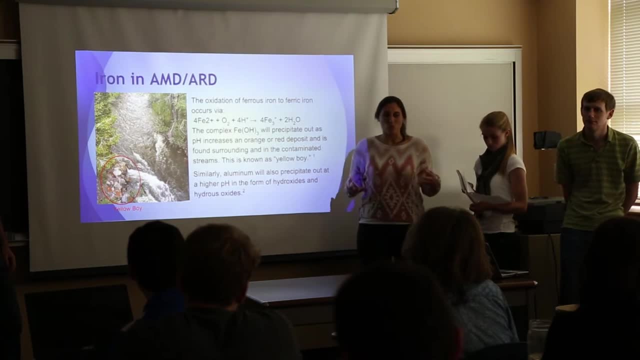 going to get together as groups hash through what the data looks like, what it means. then their groups have to produce a presentation that they'll give Friday afternoon, And so it's all a little bit accelerated. It's good for them to have to have some really short-term deadlines, But what we hope to 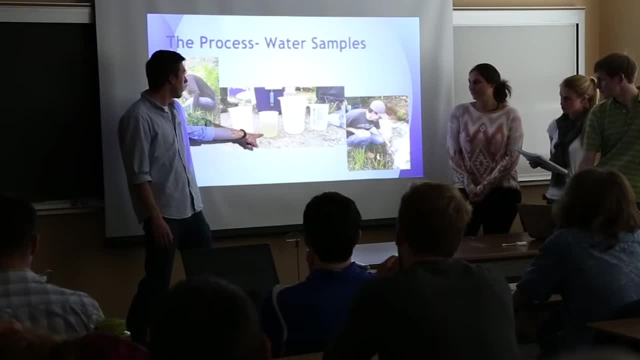 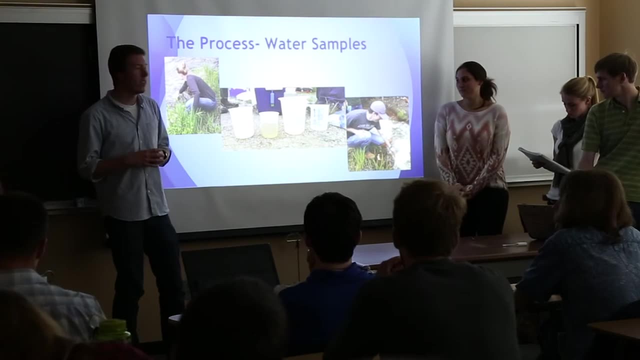 see is some good presentations on questions like: how acid is the stream? How much copper is in the stream? Is the copper above the levels that are considered safe for things like aquatic life? So we'll compare their results to what the stream standards are that.